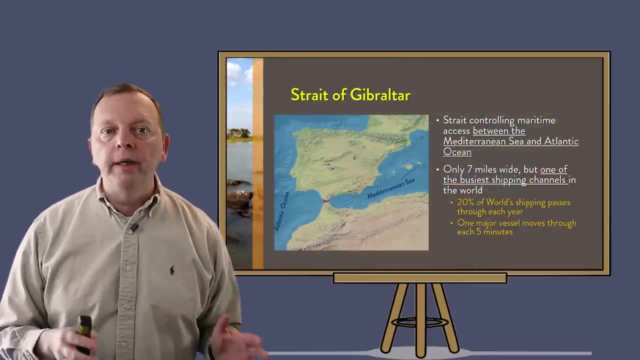 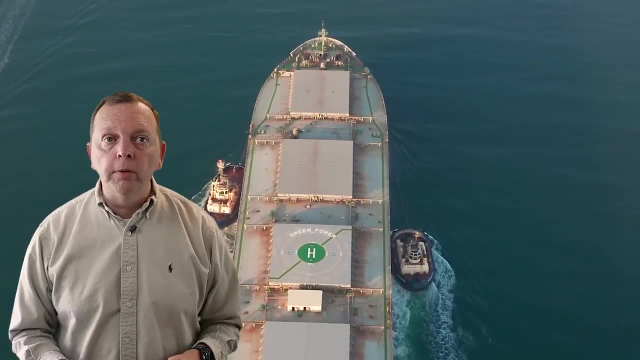 in the Mediterranean Sea we find the Strait of Gibraltar, which connects the Mediterranean Sea to the Atlantic Ocean. This choke point is only seven miles wide but is one of the busiest shipping lanes in the world. Now, 20% of the world's shipping passes through the strait each year. 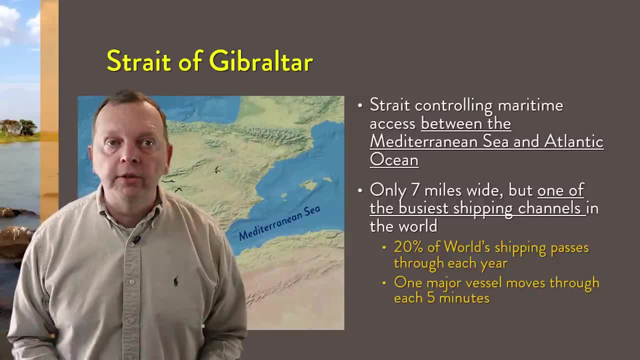 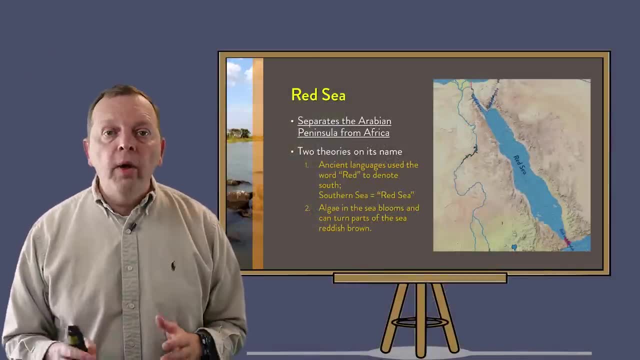 as a major ship moves through the strait every five minutes. Now separating the Middle East and Africa is the Red Sea, and there are several theories to explain the name of the sea. One theory suggests that in ancient languages the colors black, red, green and white 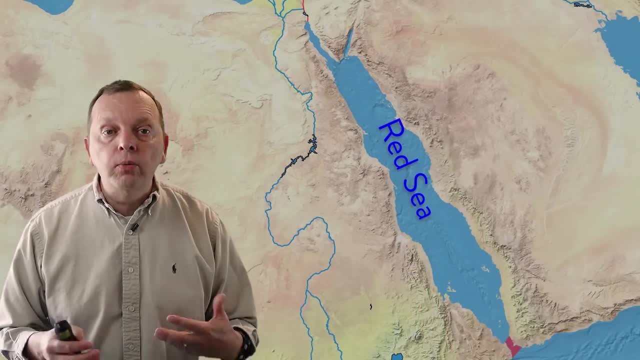 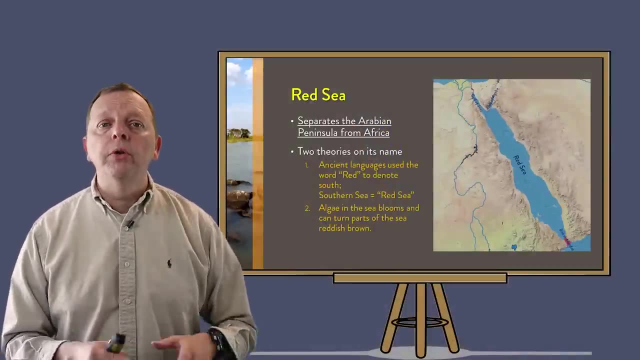 referred to the direction of the sea and the directions of north, south, east and west. so the Red Sea is essentially the sea to the south. Another theory suggests that it could be named for the algae that occasionally grows near the surface that can give parts of the Red Sea kind of a reddish-brownish color. 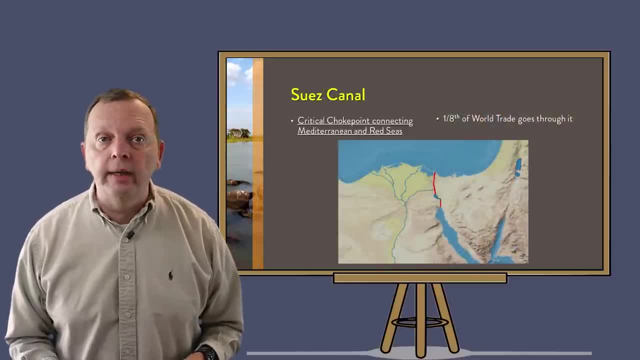 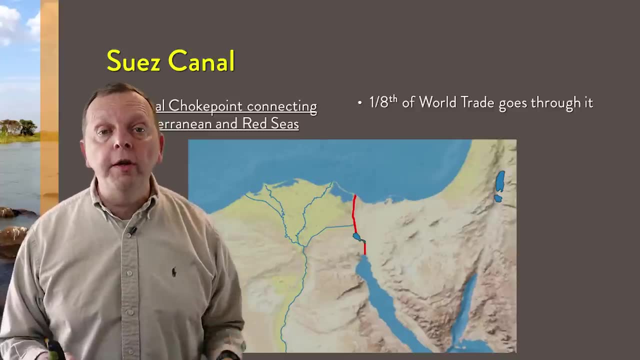 Now the Red Sea is connected to the Mediterranean Sea by the Suez Canal. Completed in 1869, the 120-mile canal cuts off about 5,500 miles of the journey from London all the way to the Arabian Peninsula. This makes the Suez Canal extremely important for training. 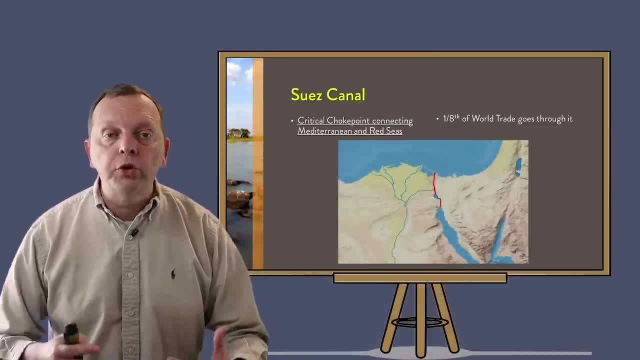 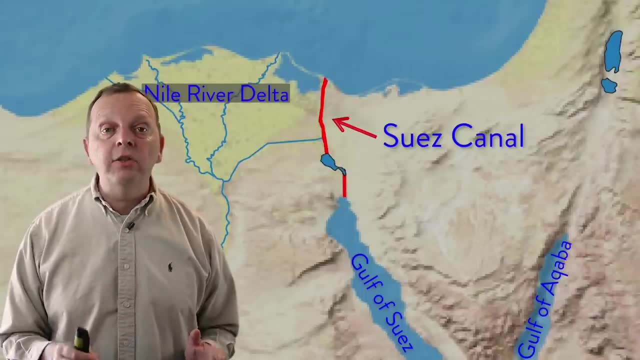 and it's also the most important part of the journey. The Suez Canal has anywhere between 9% and 13% of the world's trade passes through this canal. It is also a strategic choke point, as political or military conflicts could easily stop ships moving through the canal. 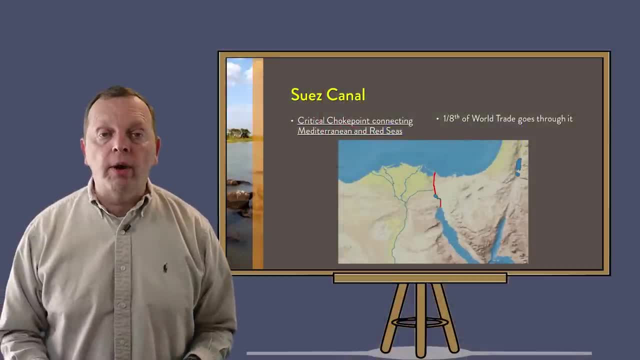 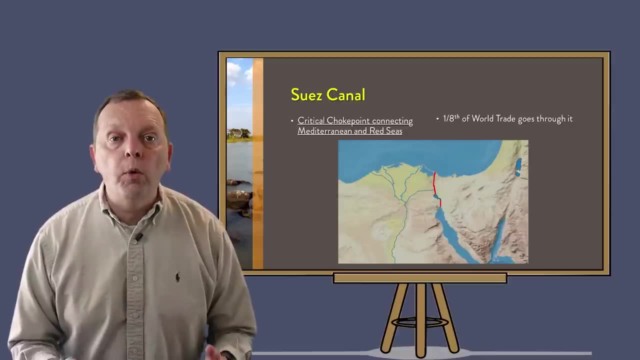 This occurred in both World War I, World War II and the Suez Crisis. that happened in 1956. But it is within Egypt's best interest to keep the canal open, as it earns over $4 billion a year levying fees against the ships that actually move through the canal. 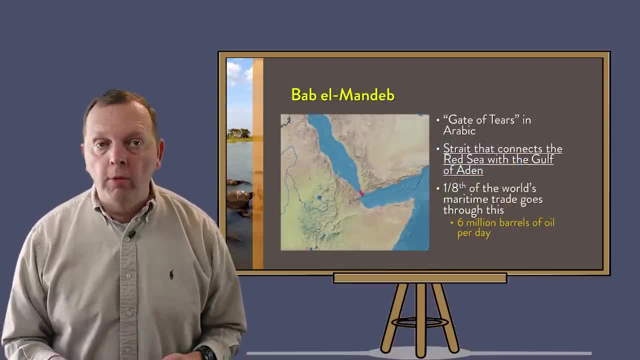 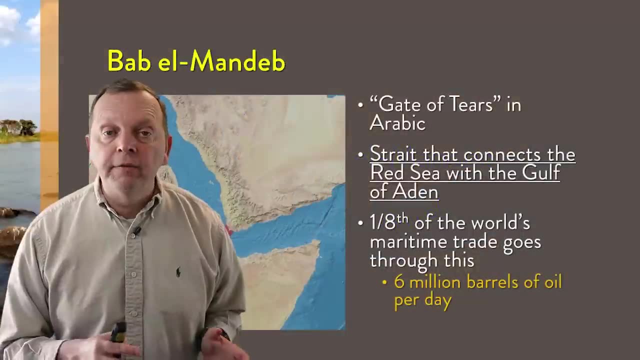 Now, to the south of the Red Sea, is another choke point: the Bab el Medeb. This strait connects the Red Sea to the Gulf of Aden. The Bab el Medeb's name actually means the Gate of Tears in Arabic, because of the dangers that early sailors faced when crossing through the strait. 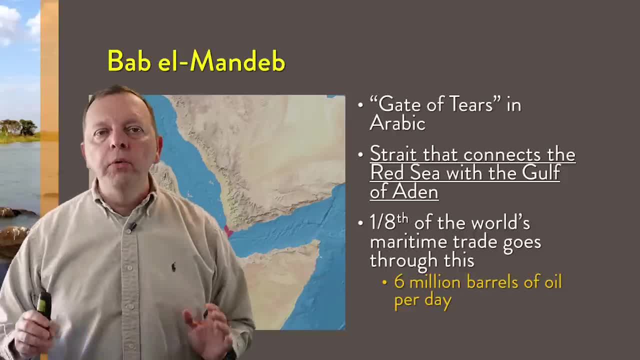 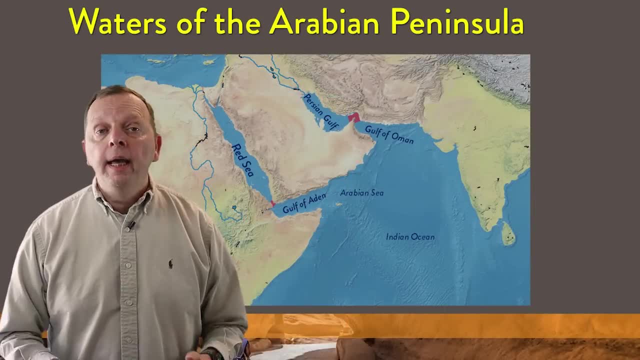 Now, like the Suez Canal, about one-eighth of the world's trade moves through the Bab el Medeb, including over 6 million barrels of oil each day. This trade opens to the Gulf of Aden, and in the late 2000s, pirates became a major concern. 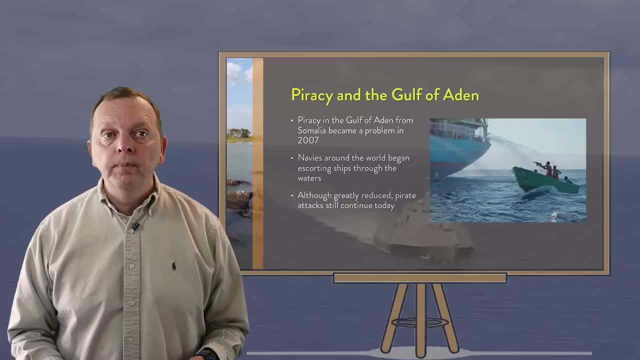 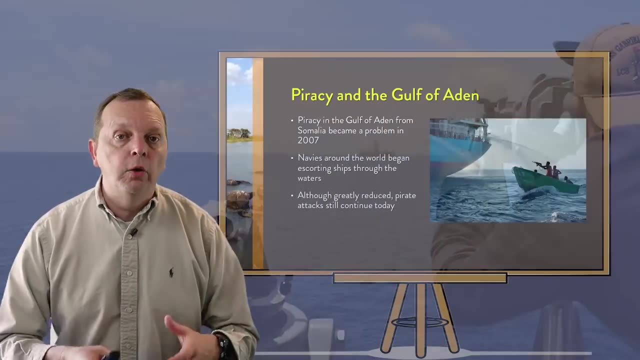 and 50 were actually being seized and hijacked every year. This caused navies from around the world, to include the United States and NATO, to begin escorting ships through the Gulf of Aden in order to keep the trade route open, And while most of the pirate activity has been reduced since 2013,. 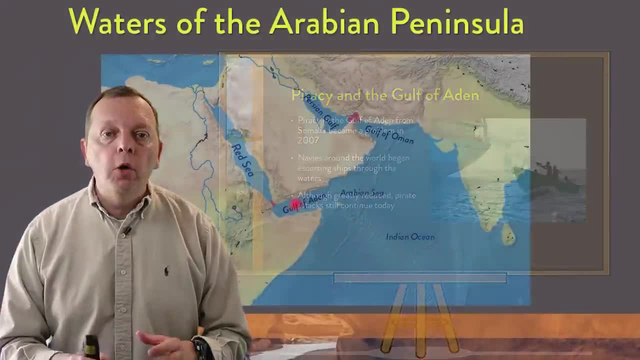 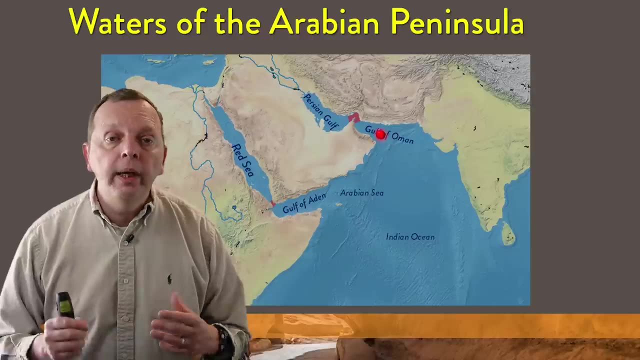 there still are events of piracy in the area today. Now the Gulf of Aden opens up into the Arabian Sea, which is a sea in the Indian Ocean. Now, as we move to the eastern side of the Arabian Peninsula, we enter the Gulf of Oman and, once again, 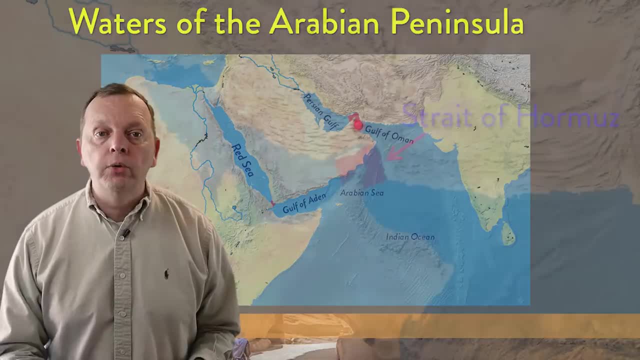 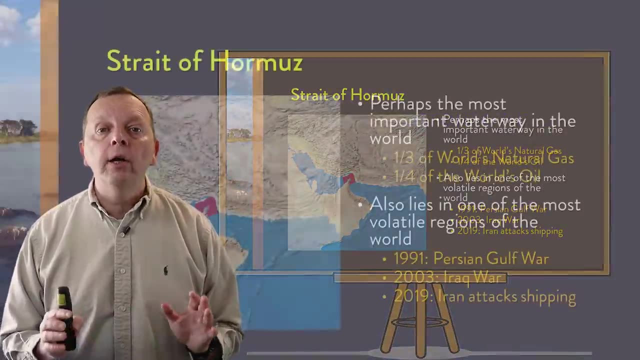 we get ready to go through another choke point. This one is the Strait of Hormuz. This choke point is arguably the most important waterway in the world, as one-third of the world's natural gas and a quarter of its oil must actually pass through. 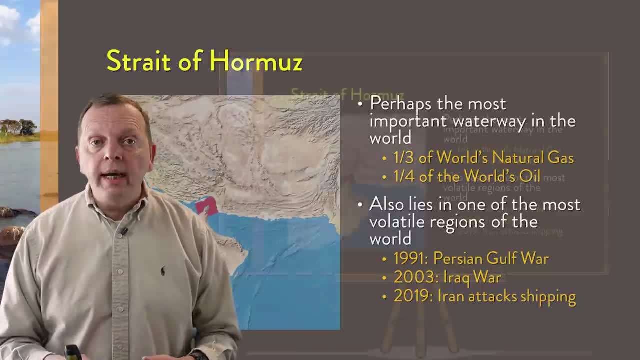 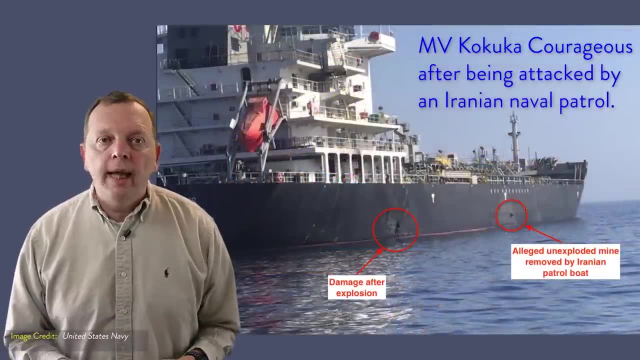 the strait Now, considering that it is only 21 miles wide and lies in the middle of one of the world's most volatile regions. this trade has been very successful. It has been blocked several times in recent history, Even as recently as 2019, Iran was attacking selected ships that were passing through the 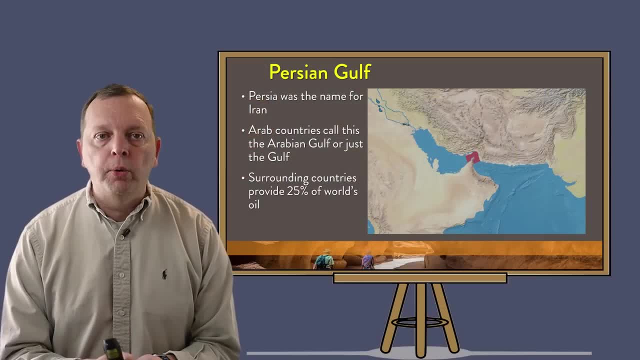 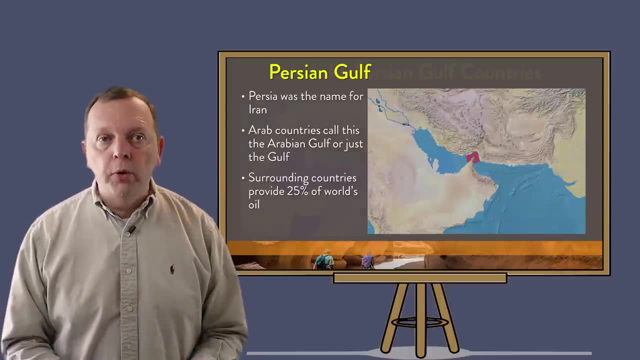 strait. Now, once through the Strait of Hormuz, we find ourselves in the Persian Gulf, although several Arab governments will call this the Arabian Gulf or just the Gulf, And it is the countries surrounding the Persian Gulf that over 25% of the world's oil comes from. 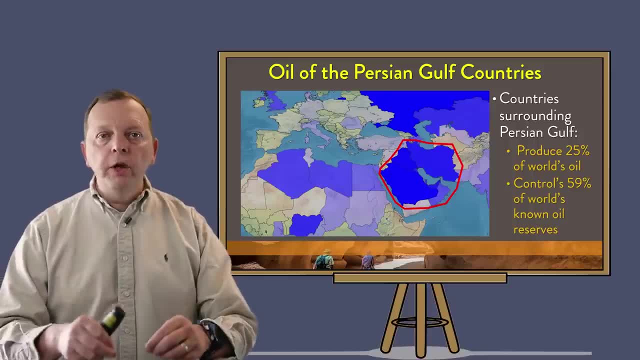 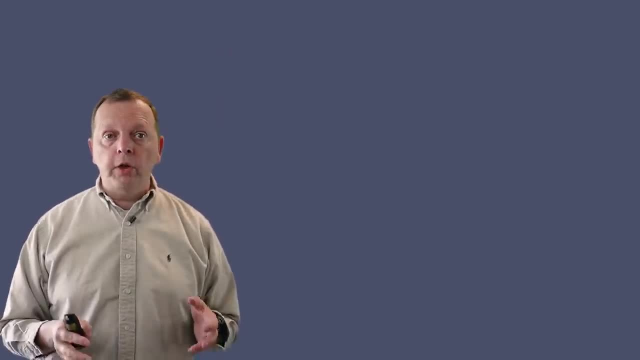 In fact, nearly two-thirds of the world's known oil reserves are found in this region, making this a very important region to the world's economy. Unfortunately, it has also been the scene of many of the world's most recent conflicts, to include the 1991 Gulf War and the war in Iraq that started in 2003.. 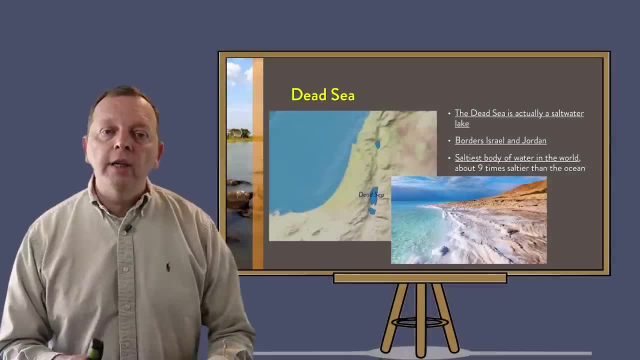 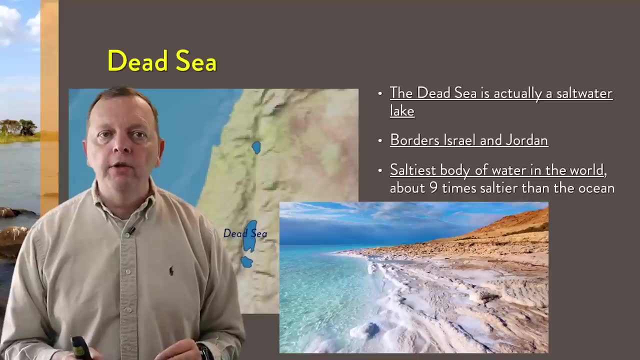 Now there is one other sea that we'll have to look at, which is the Dead Sea that is found in between Jordan and Israel. The Dead Sea is one of the saltiest bodies of water in the world. Now let's put this in perspective. 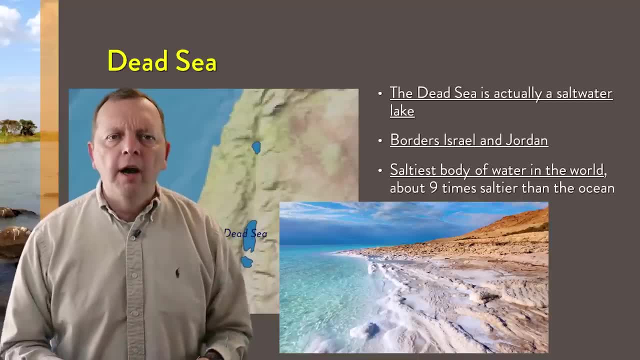 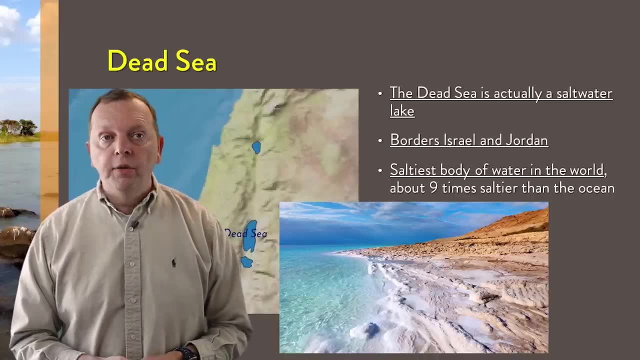 The salt in the world's oceans are about three and a half percent of its weight. The Dead Sea, however, has over nine times as much salt, at about 33.7% of its weight. The fact that nothing except for bacteria can survive in such salty water. 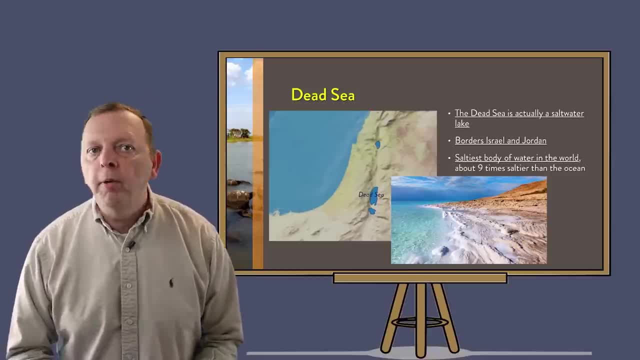 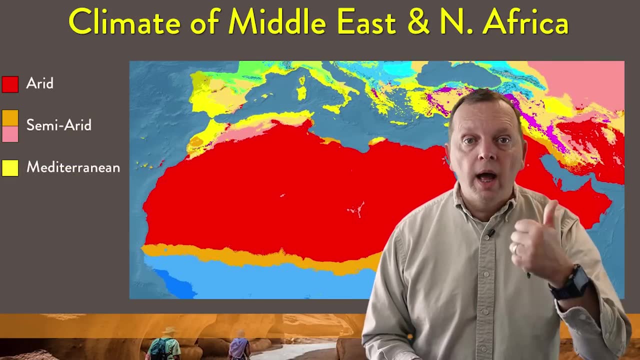 is the reason for the sea's name: the Dead Sea. Now, before we talk about the region's landforms, let's take a look at its climate. We could probably best describe the region's climate in just two words: hot and dry. 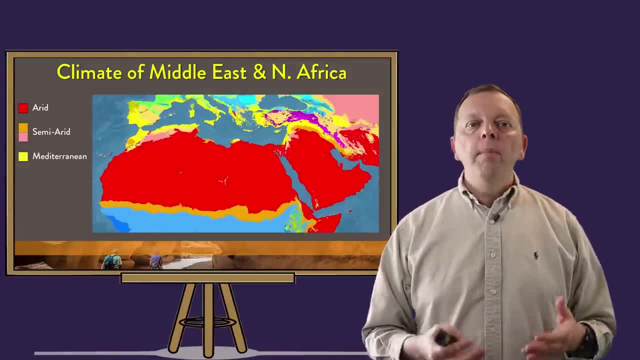 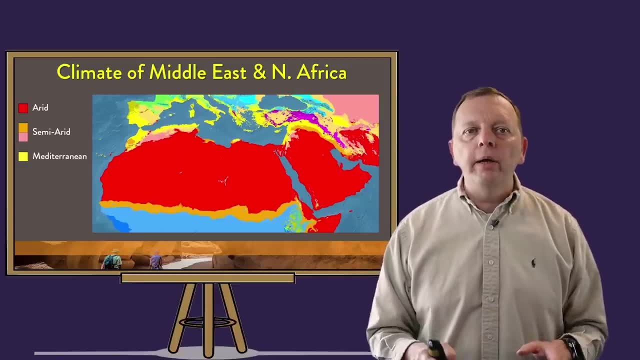 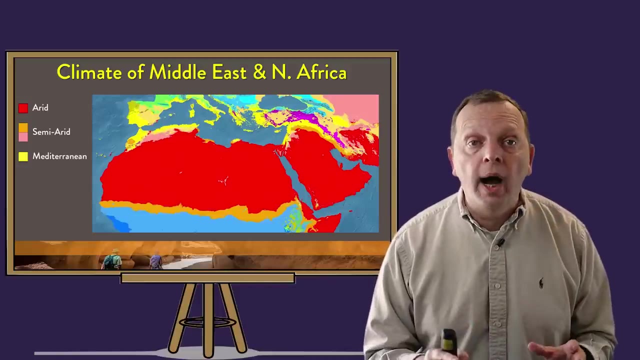 Now from personal experience- my first time in Iraq in 2003,- my personal thermometer read 132 degrees. Now that was probably incorrect, but the temperatures in Iraq and other areas in the Middle East routinely go over 120.. In 2016,, Kuwait and southern Iraq had official highs of 129 degrees. 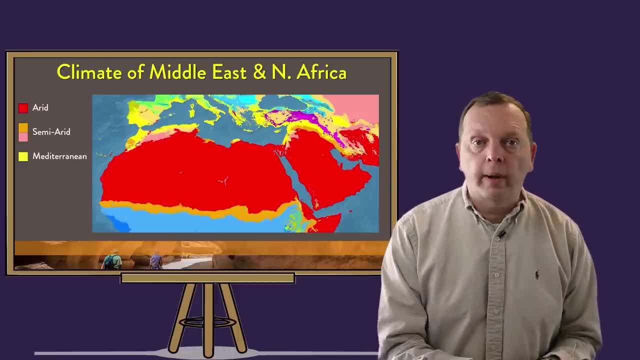 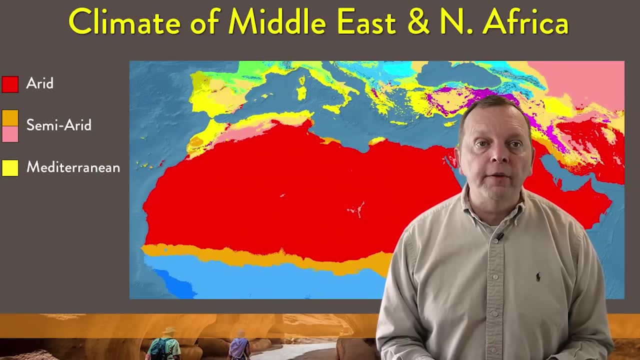 Now, as this climate map shows, despite the mountainous areas of Iran and Turkey and the coastal regions surrounding the Mediterranean Sea, which has a Mediterranean climate, the dominant climate in Middle East and North Africa is a dry, arid climate. This means deserts. 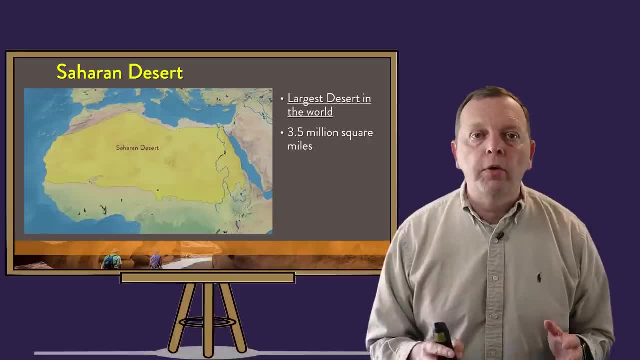 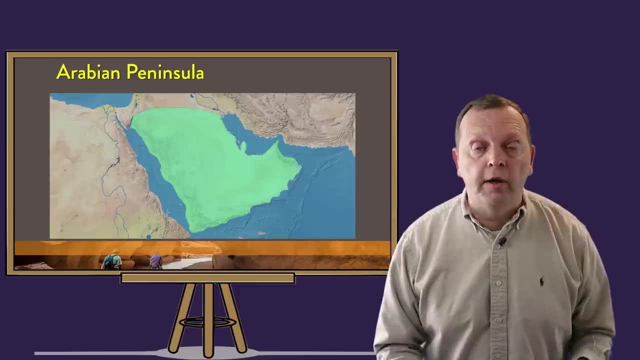 The largest desert in the world is the Sahara Desert, which measures over 3.5 million square miles and stretches across northern Africa, The Arabian Peninsula, but is also nearly fully covered by deserts. The Arabian Desert is the third largest desert in the world. 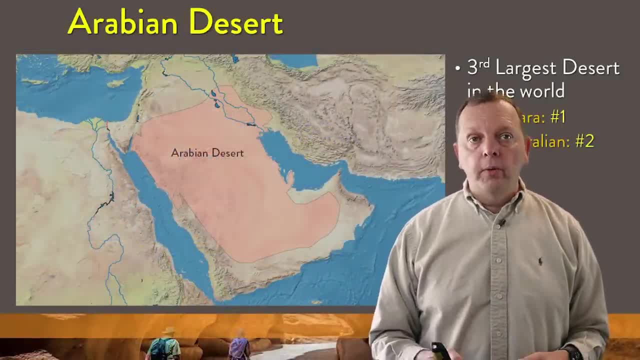 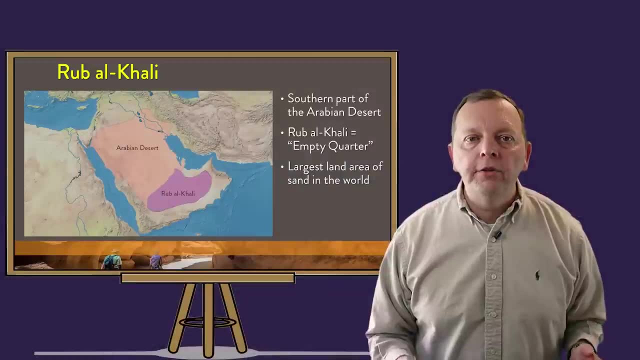 after the Sahara and the Australian Deserts, The southern third of the Arabian Desert is known as the Rub' al Khali, or the Empty Quarter. The Rub' al Khali is also the largest area of sand in the world. Now let me put this in perspective. 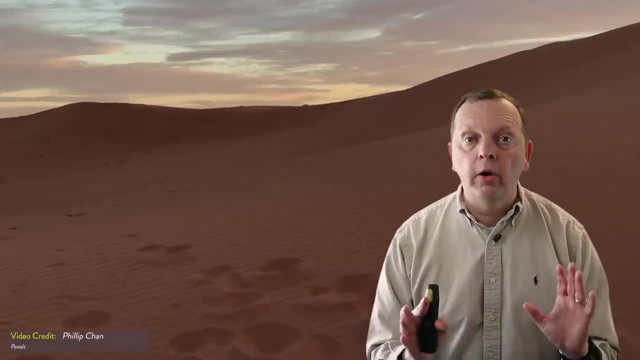 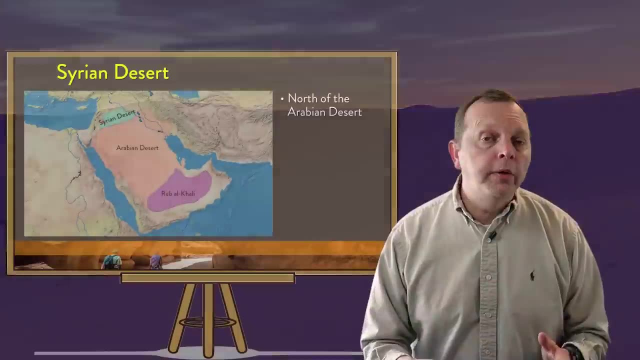 The Rub' al Khali has half the amount of sand that the entire Sahara Desert has, despite the fact that the Sahara Desert is actually 16-times larger than the Rub' al Khali. Now the Montalbany Desert No. 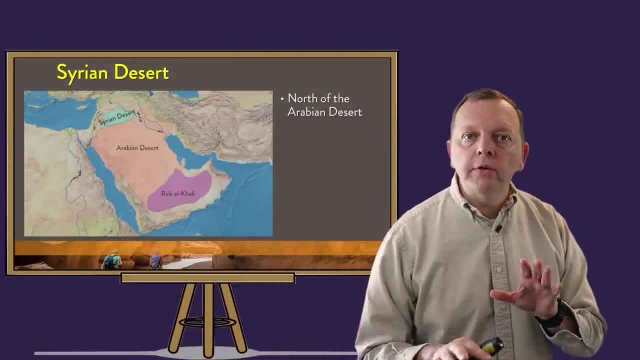 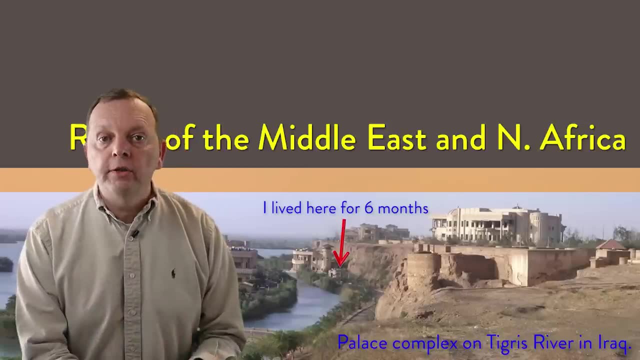 of the Arabian desert, we have the Syrian desert, and if we go down to the southern portion of the country of Israel, we find the Negev desert. Now there are rivers that flow through these deserts. Now, more than just providing scarce water to the region, these rivers also have been the home of 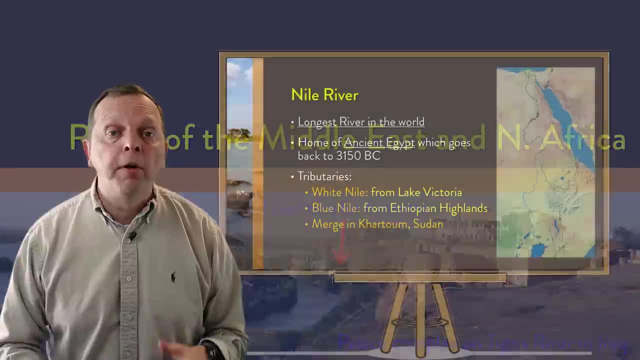 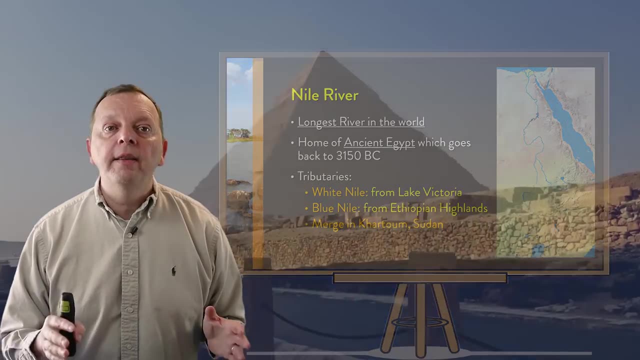 the world's earliest cities and empires. For example, flowing through Egypt, we have the Nile, which is the world's longest river, Now flowing from the south to the north. it is along the Nile's banks that the ancient Egyptian civilization and their pyramids are found. The Nile begins down in. 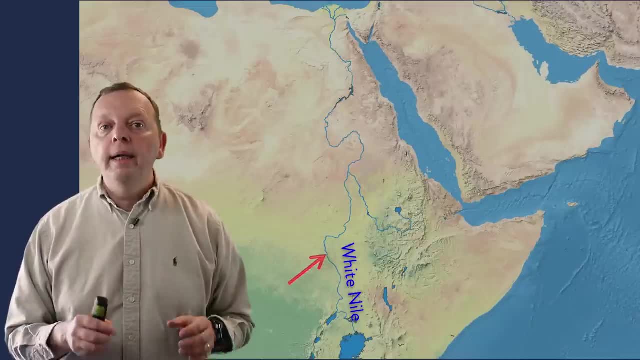 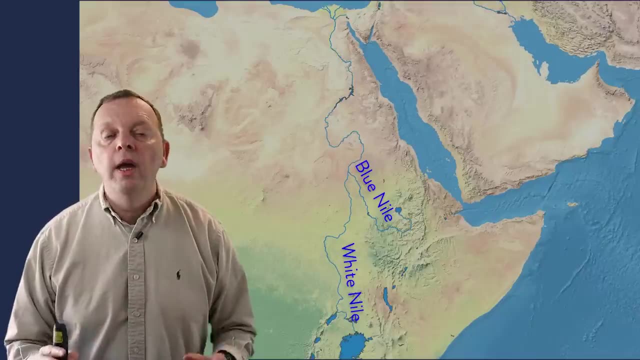 the south: in Uganda, where Lake Victoria feeds the White Nile, and in Ethiopia, where the waters flowing out of the Ethiopian highlands feeds into the Blue Nile. Now the Blue and White Nile tributaries continue flowing northward until they merge in Kharkoum, Sudan, and become the Nile River. 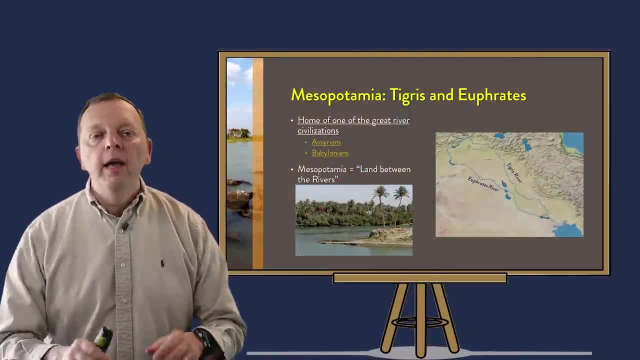 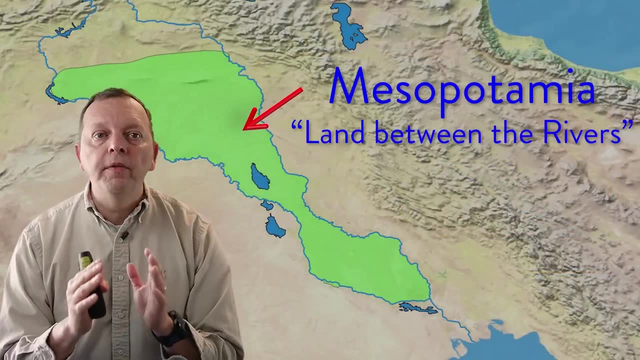 Now in the Middle East. the Euphrates and Tigris rivers begin in Turkey and flow south through Syria and Iraq before entering into the Persian Gulf. It is in between these rivers that we find the home of the ancient Mesopotamian civilization of the Assyrians, and 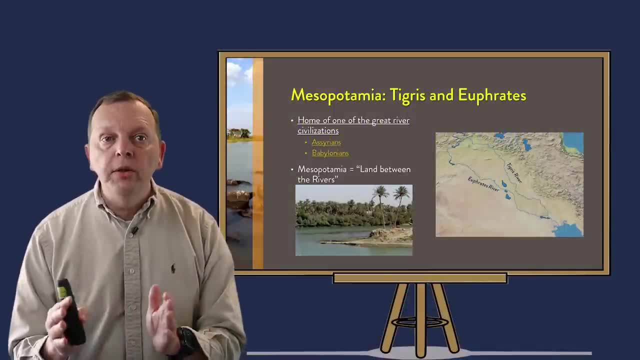 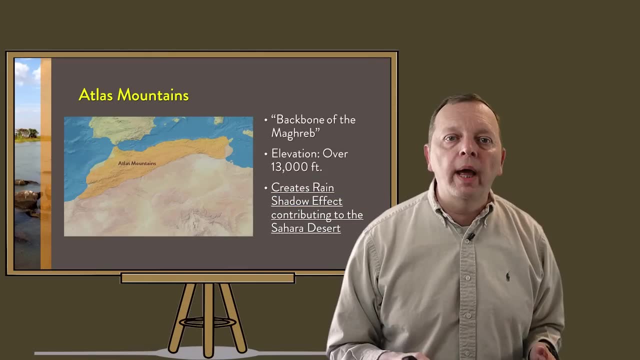 the Babylonians. See the name. Mesopotamia actually means land between the rivers in ancient Greek. Then there are the mountains, and the northwest portion of northern Africa are the Atlas Mountains, which are also known as the backbone of the Maghreb. The Maghreb is the western region of the 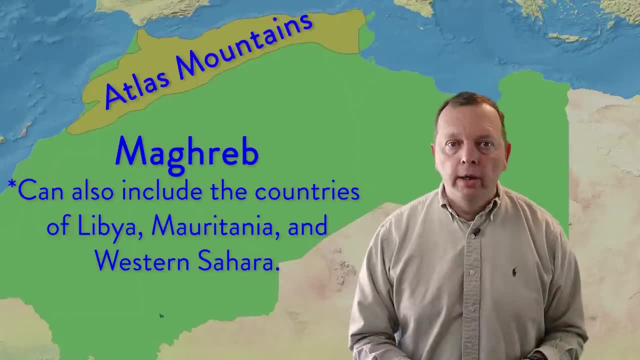 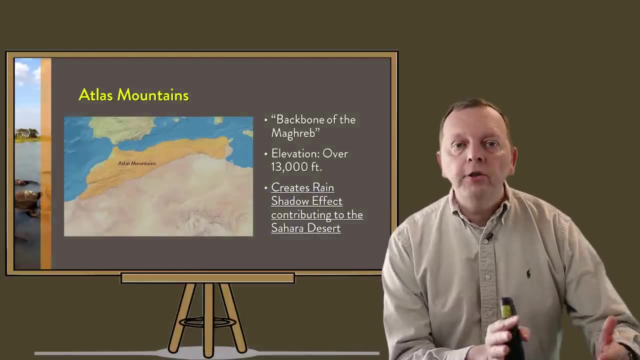 Arab world and includes the countries of Morocco, Algeria and Tunisia. The Atlas Mountains are pretty decent-sized mountains, rising up to about 13,000 feet, and through the rain shuttle effect they'd actually help blocking the precipitation from the Atlantic Ocean from coming to the Sahara Desert. Now the 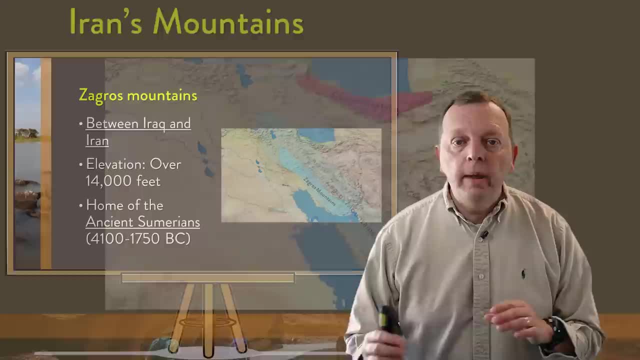 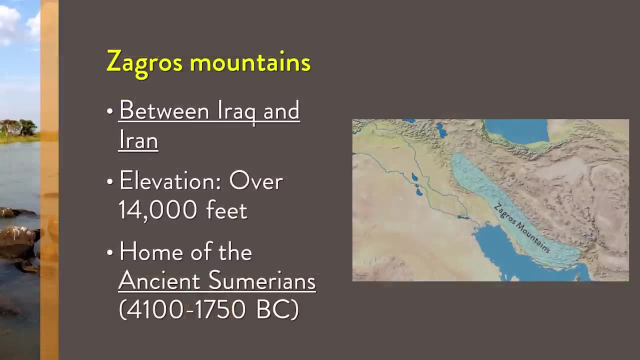 two other mountain ranges we'll talk about are both in Iran. Now in between Iran and Iraq, and stretching up to Turkey, we find the Zagros Mountains, which stretches up to 14,000 feet, and it was within the Zagros Mountains that the ancient Sumerian civilization. 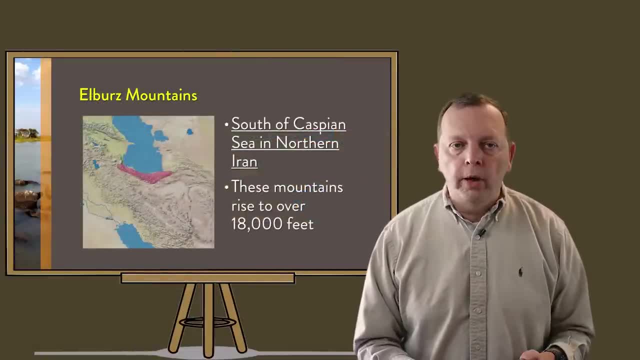 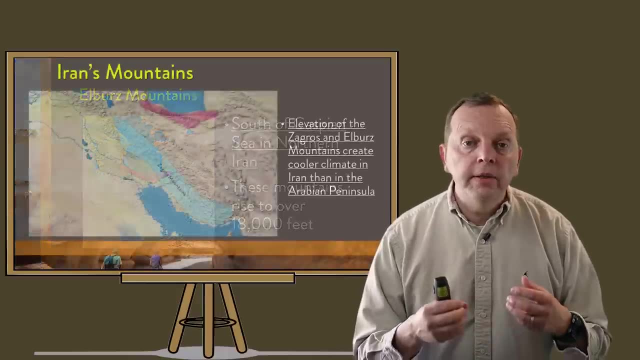 made their home. The second mountain range in Iran is the Elbrus Mountains, which lies to the south of the Caspian Sea in northern Iran and climbed to over 18,000 feet. Now it is the Zagros and Elbrus Mountains that gives Iran an overall cooler climate than what 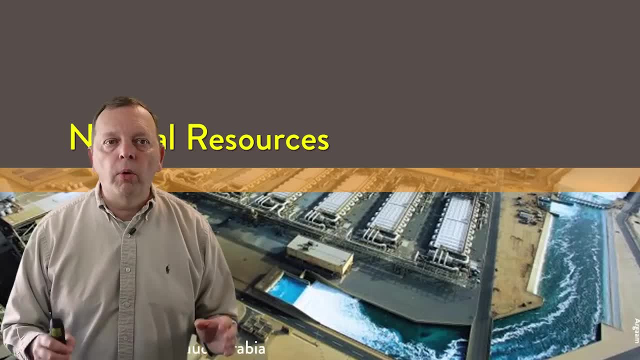 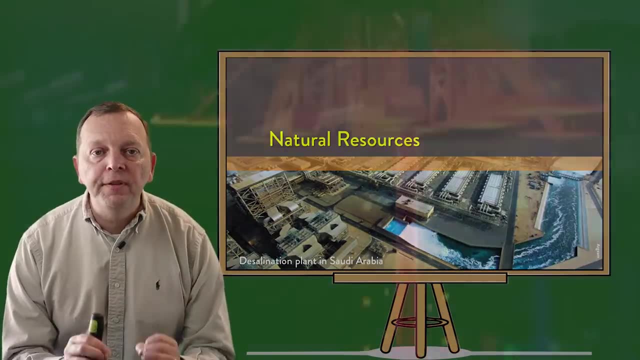 we find in the rest of the Middle East. Now. we have already discussed the importance of oil in the Middle East and North Africa. Despite only having six percent of the world's population, this region has 59 percent of the proven oil reserves in the world and 45 percent of the 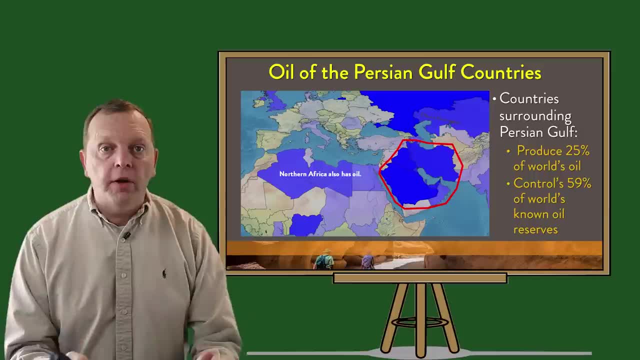 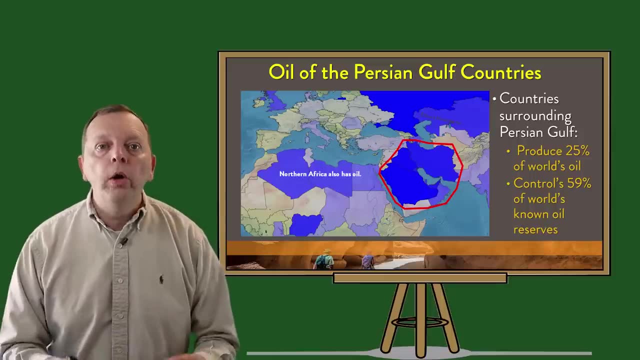 proven natural gas reserves. So, in a world that still runs on fossil fuels, this makes the region extremely important to the world's economies. Moreover, for the oil producing countries in the Middle East, oil is the major driver of their economy. They are also fortunate that not. 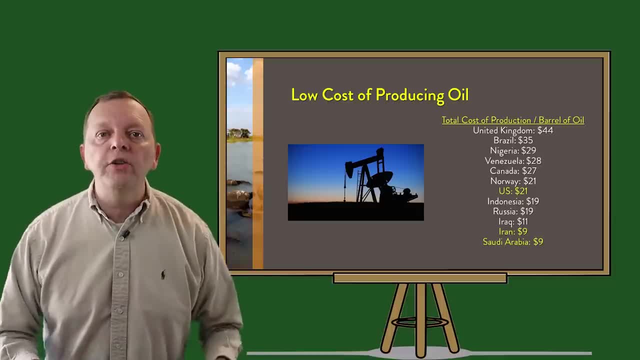 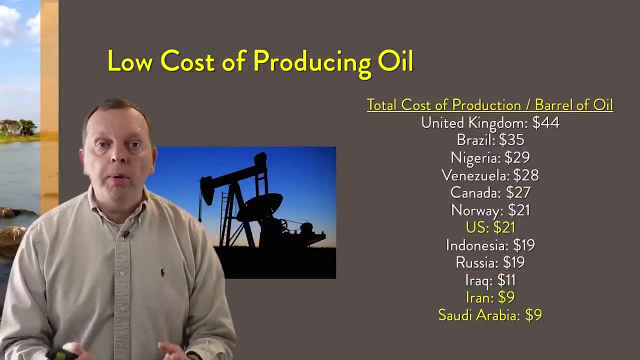 only do they have lots of oil. unlike other places in the world, their oil is actually much easier. thus it is much cheaper to be able to get to and drill. See, it only costs Saudi Arabia nine dollars to be able to pump one barrel of oil. However, in the United States that actually costs as much as 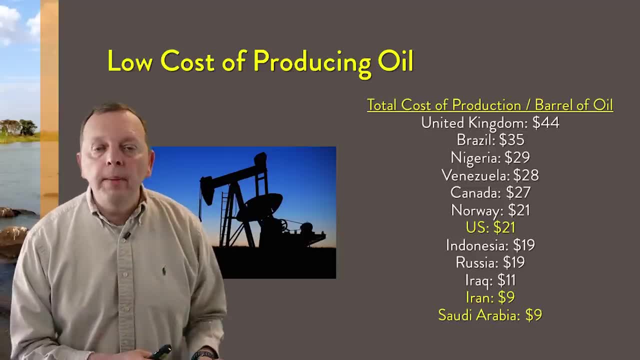 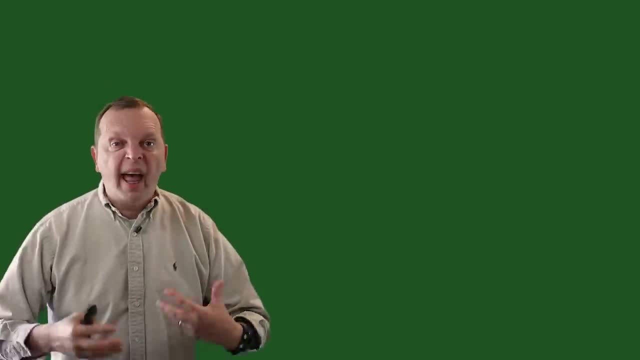 twenty one dollars. This means that Saudi Arabia easily profits ten dollars more a barrel than in the United States or other places in the world. Now, while oil is so important to the region, because of how much oil there is, the other most important resource in the region is important. 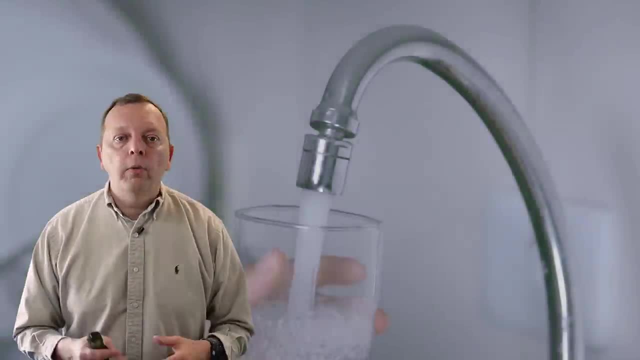 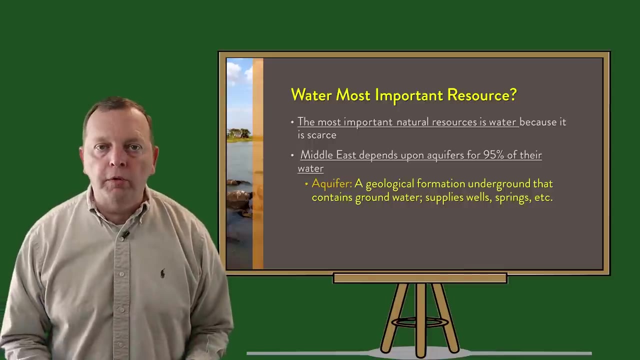 because how little there is, and that is water. Now, remember, the people of the region are only six percent of the world's population, but it only has about one percent of the world's renewable fresh water. Now, because most of the surface in the Middle East and North Africa are deserts. 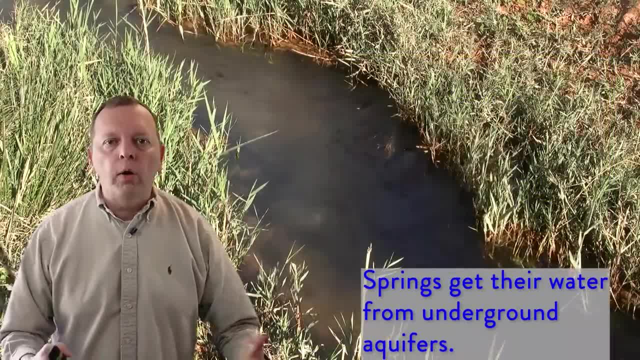 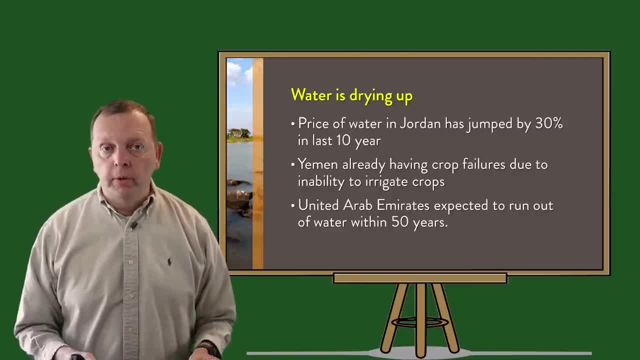 most people have to rely upon aquifers or lakes of underwater water for their drinking water. However, the water in the aquifers is quickly being used up. This is causing many problems in the Middle East. In Jordan, the price of water has risen by thirty percent just in the last ten. 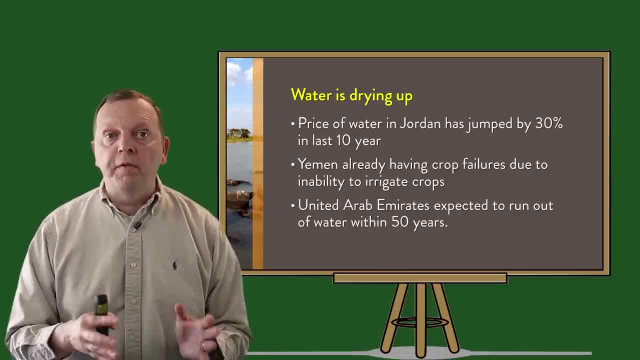 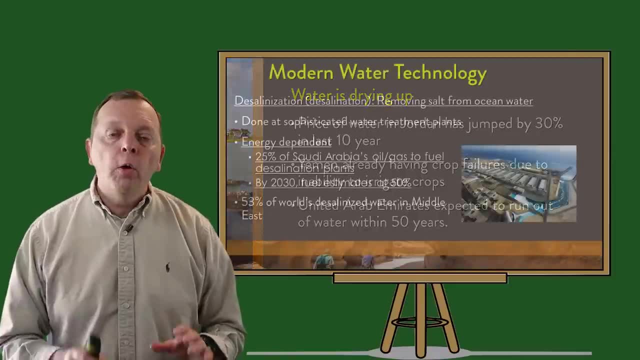 years. Yemen is already suffering crop failures, as water is not available for farming, and even the super wealthy country of the United Arab Emirates is estimated to run out of water in the next 50 years. Now one solution that Arabs are turning to is desalination plants, In fact, 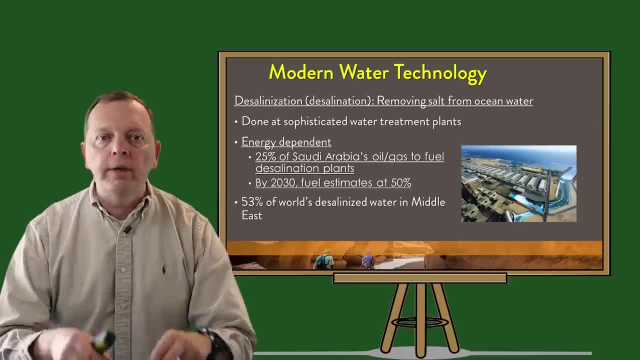 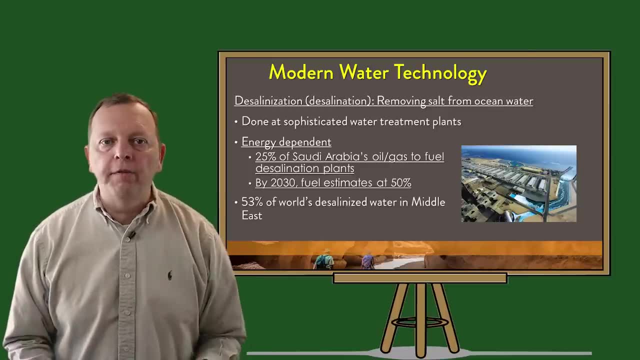 70 percent of the world's desalination plants are actually found in the Middle East. What these plants do is they take water from the surrounding seas and they separate the salt from the water, providing fresh water. Today, 50 percent of the drinking water in Saudi Arabia comes from these. 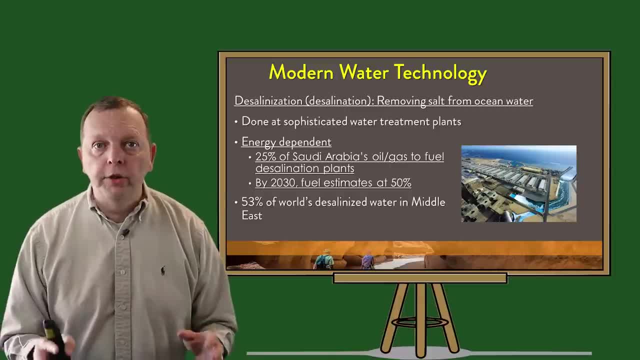 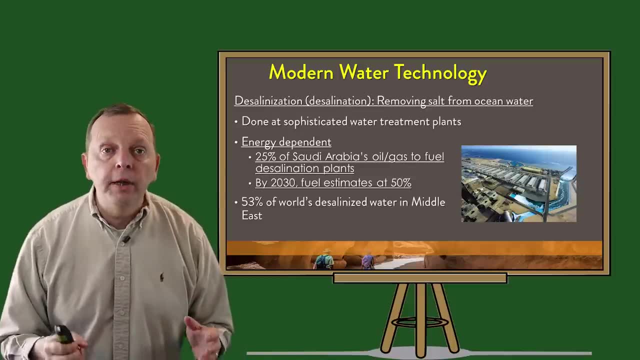 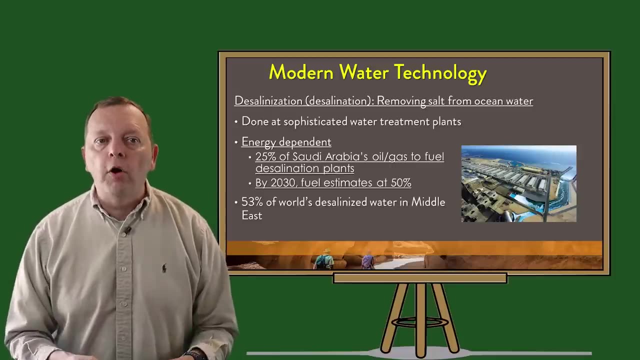 desalination plants. However, these plants take a lot of energy to run, so much that 25 percent of Saudi Arabia's oil and gas products actually are used to run these plants, And by 2030, some estimate that 50 percent of Saudi Arabia's oil will be used to create drinkable water for its people and farms. 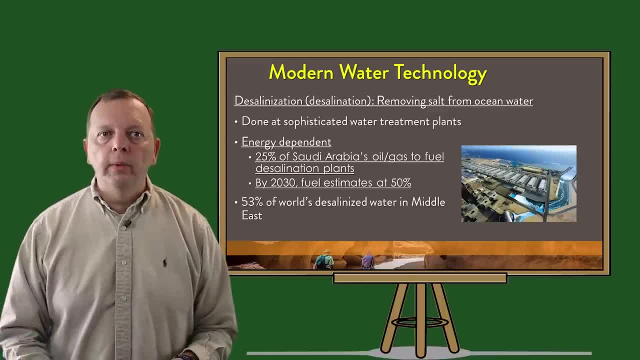 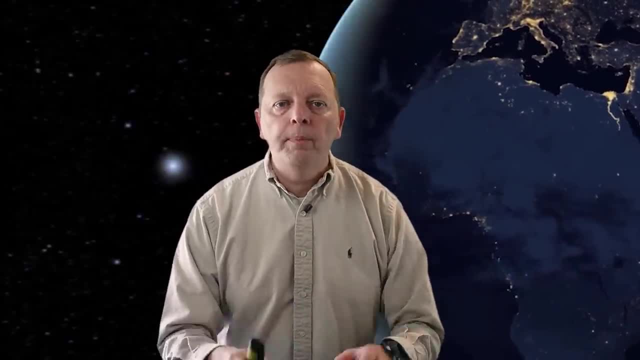 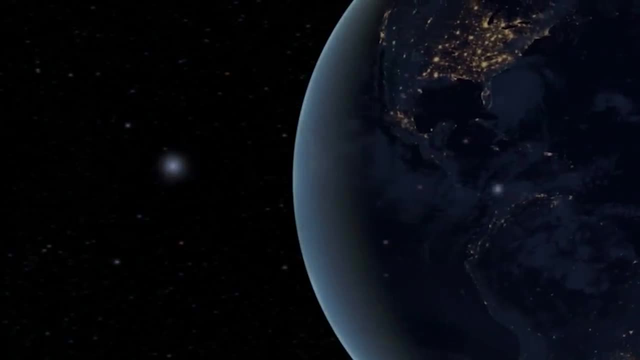 Water is literally becoming as valuable as oil in the Middle East. All right, that is the physical geography of the Middle East, North Africa and our next lessons. we'll start looking at the culture and the people of the region. Until then, keep on learning.